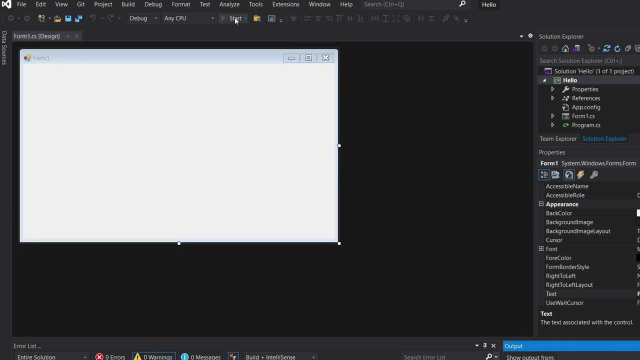 And It is When you start the program from here. it will appear on the screen and you can add things inside of it. You can change the behavior of it, You can change a lot of things. So here you can resize it. 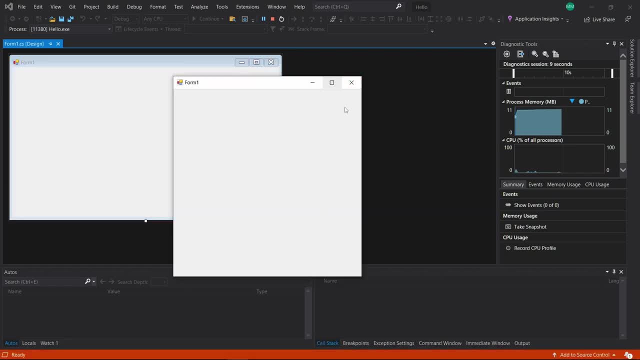 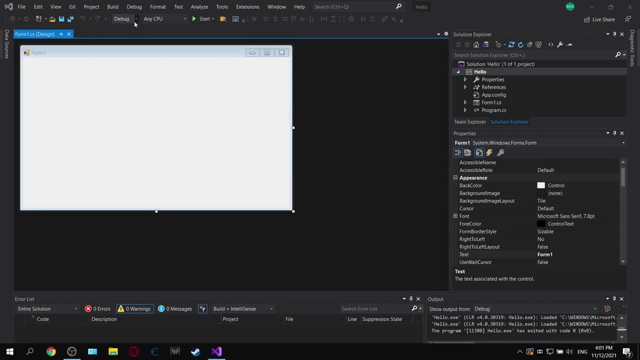 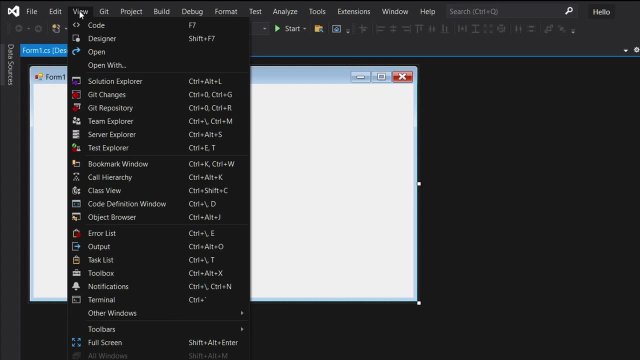 You can minimize And then you can also make it bigger. So, and then now we can add functionality to the form. Okay, So to add tools to the form, you want to go to the View tab and then you want to select the Toolbox. 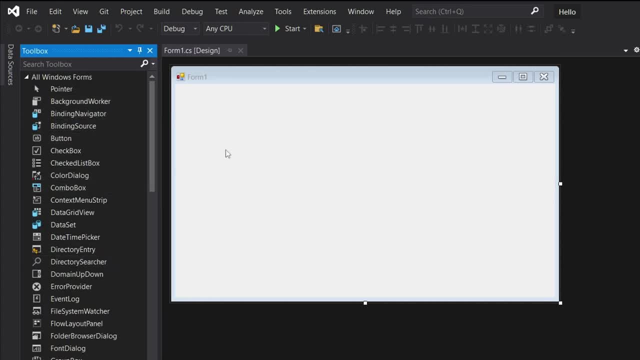 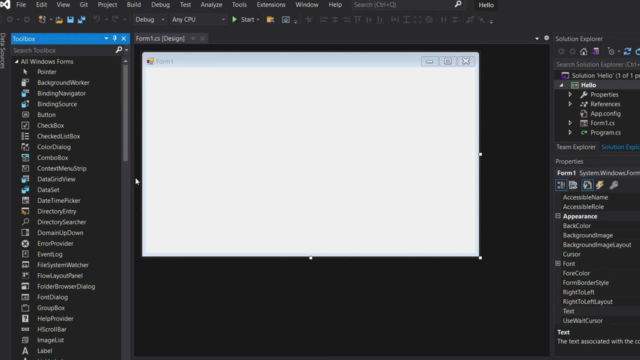 Here you will find everything that you want. You need to create the app that you want. So we are going to use buttons and we are going to use labels to print something on the screen using the Windows Forms. Okay, So first we want one button. 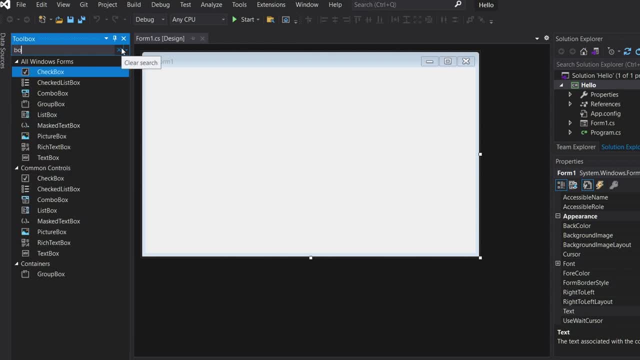 So here you can find the tools, You can also search for them. So here you can find the tools, You can also search for them. So here you can find the tools, You can also search for them. 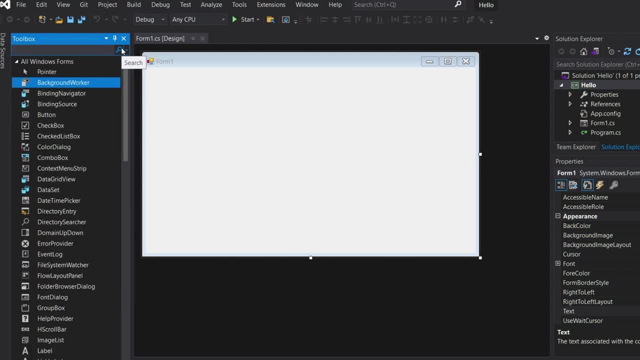 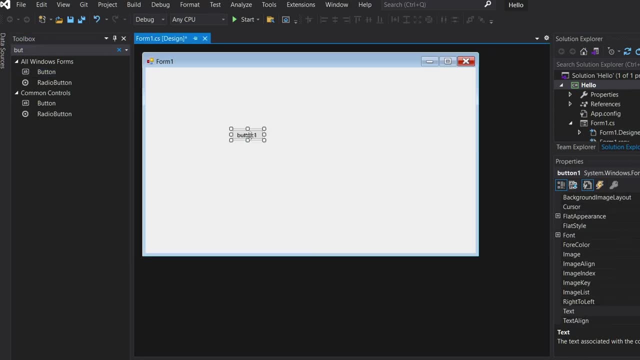 If you want a button, if you want a label, if you want everything, anything you can type it here. So a button, I'm going to select a button and then I'm going to put it here. You can put it wherever you want. 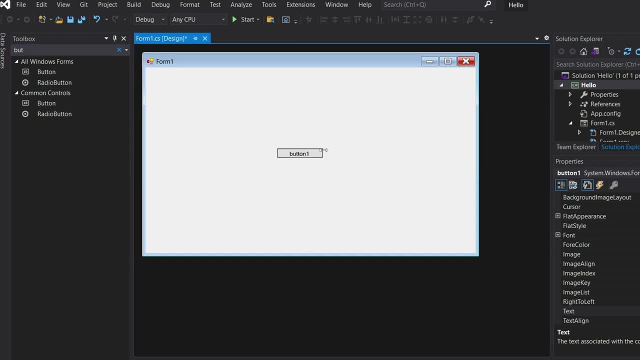 And then you can also change the size of it. Okay, We'll talk about that later. So, and then also, I want to add a label. So I'm going to search for a label. So we want a label. 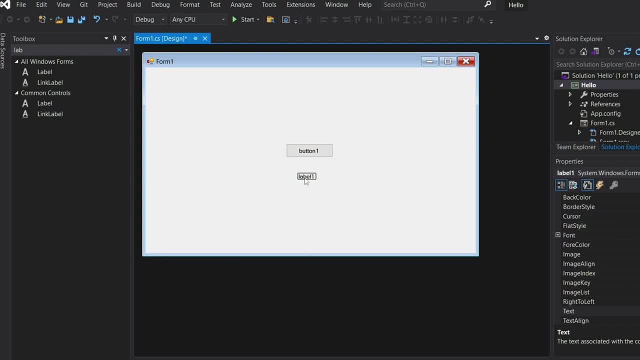 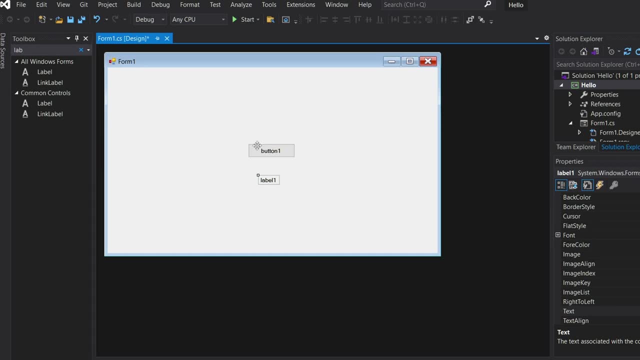 This label will only display text. It doesn't do anything, but just displays text. Okay, So let's make it where we, if we press on this button here, we will make it that when we press on this button, it will change the text here. 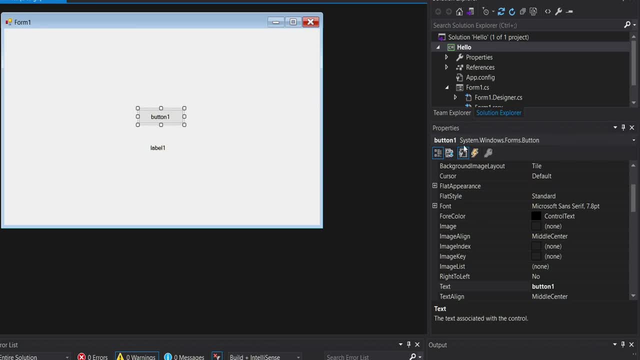 Okay, So first you can see here in this step over here you'll find properties, and if you don't see this here, you can Right-click on this and then you can select properties. It will show over here. 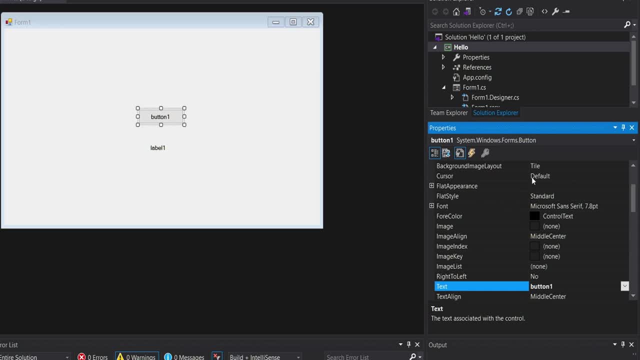 Okay, And then you want to Here you can change the properties of this button here. So let's change the background of the button so it is different than the screen. Okay, So they are very similar, So let's change the background of the font. 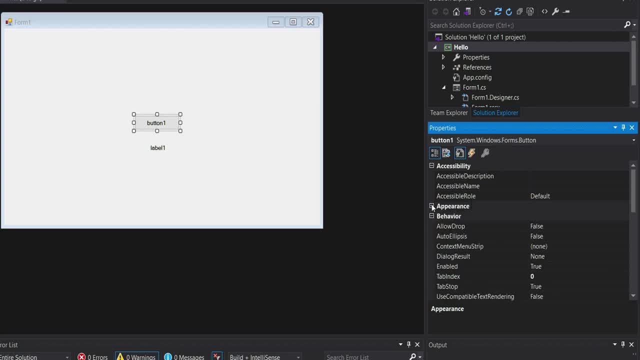 So in the appearance section- Okay, You want to. you want to go to the background color, back color, and then you can change it to whatever you want. So I am going to change this to something a bit different. Okay, that's not good. 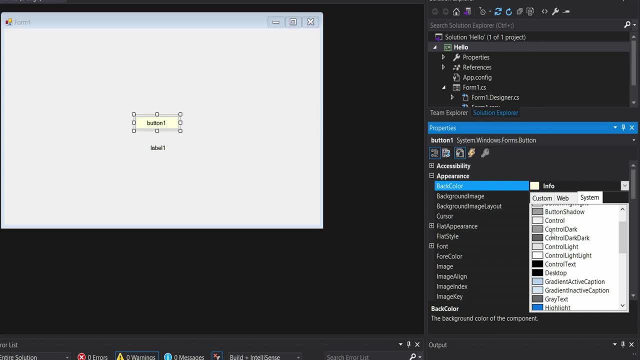 I don't like that. Let's change it to this: Okay, this is much better. You can see the font much clearer, So you can also change. Let's change the whatever this says. So here it says: button one: 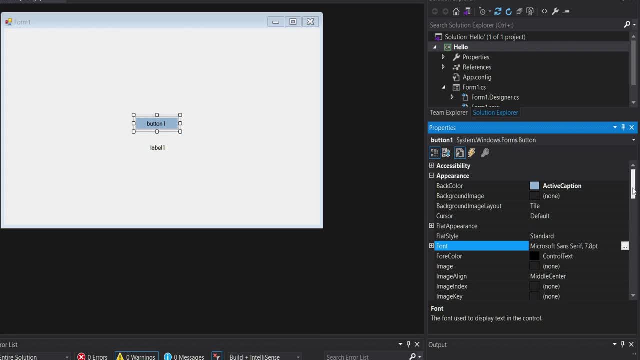 So we can change that from the under the font tab. here under the font You can select the color of the text and then you can also change the text. So in the text tab here you need to select and type. 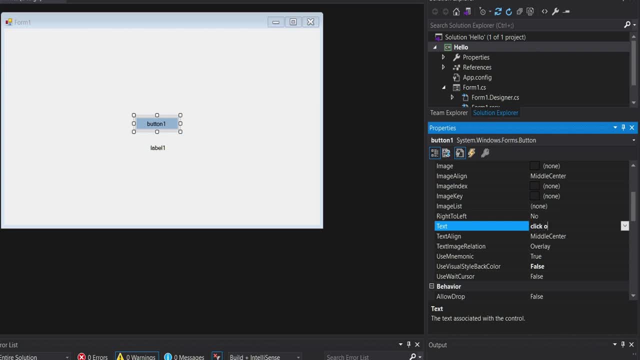 Okay, let's call this button: click on me. Okay, So we will inform the user to click on the button. And then, when we click on this button, we will change the whatever this label here says. Okay, So you can also change the color of the font. 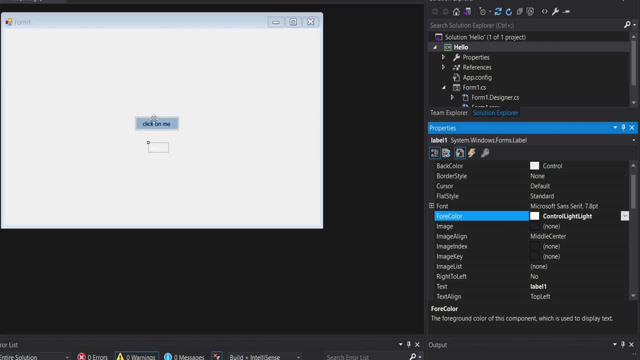 You can change it to white, Not here. I selected the label. Go back, Okay, Okay, So now. Now here you can change this color. So let's change it to white. You see, But it doesn't show very well. 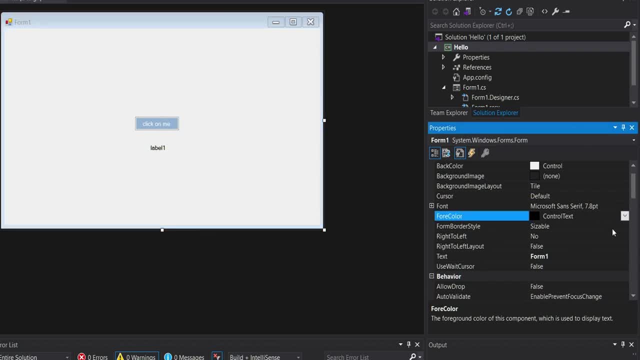 So you can. just I want to keep it black, Not that black, Not label. I keep pressing on the label. Okay, So we will select that And then we are going to make it bold. It appears much better. 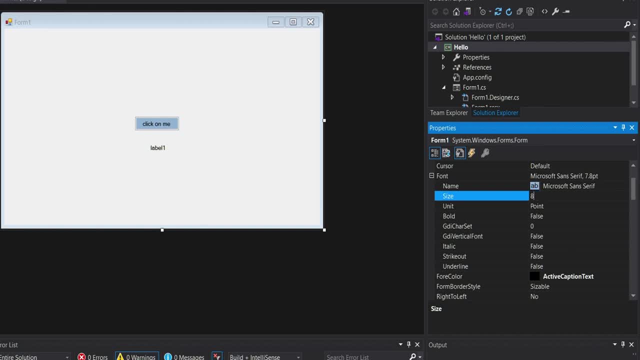 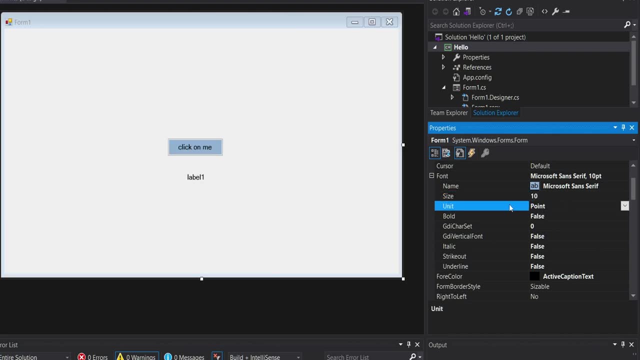 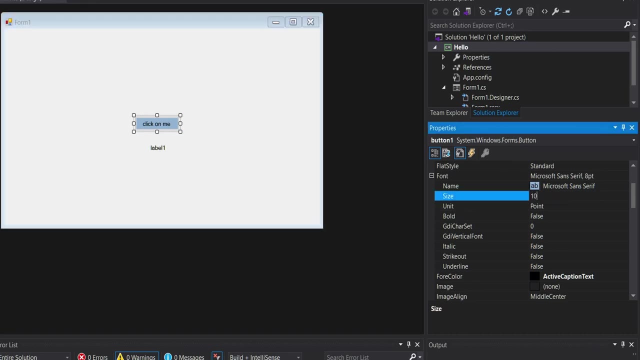 Okay, So we can also make it a bit bigger. So let's make it 8. Or 10. 10 is enough. Nope, I was selecting the form, So 10. Okay, And then we want it to be bold. 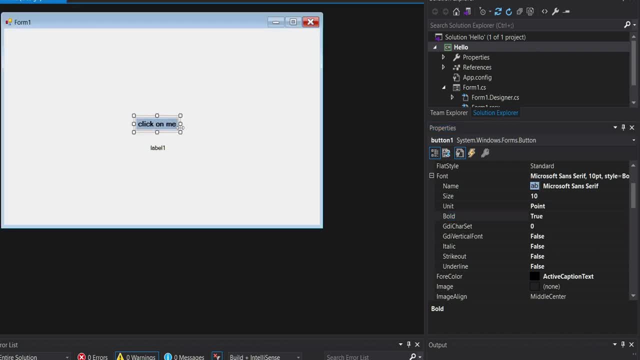 So bold here is true. So now we can make it. We made it bold And it's much clearer, Much more clearer. Let me change the font, The text, a little bit. I'll make it uppercase. Go to text. 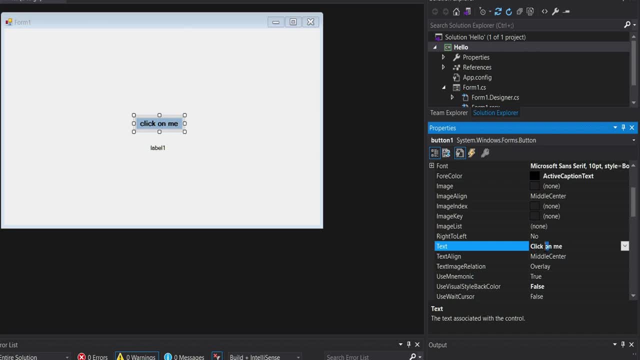 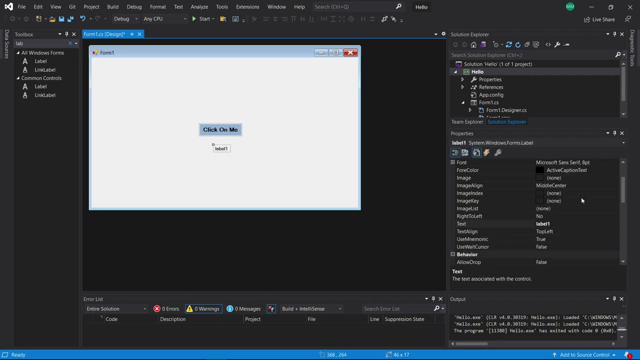 Let's make it uppercase. So uppercase on me, Everything uppercase. Okay, Click on me. That's good Enough. Let's make it a little bit bigger, Okay. And then we want to change this font to be nothing. 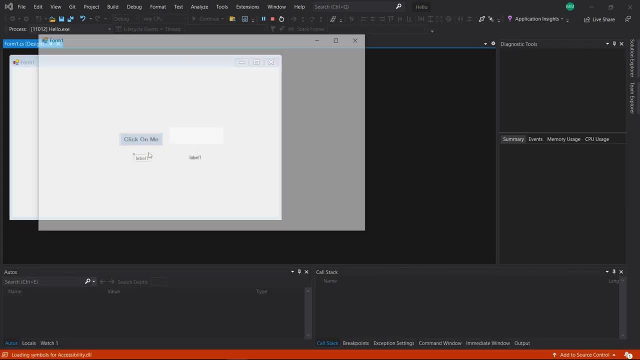 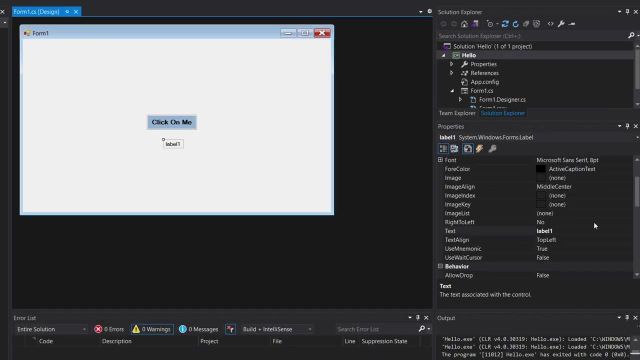 So if I run the program here, it will always appear. This text will always appear. So we don't want this to happen. So if we want it to not appear, you can just make the text not say anything And it will disappear. 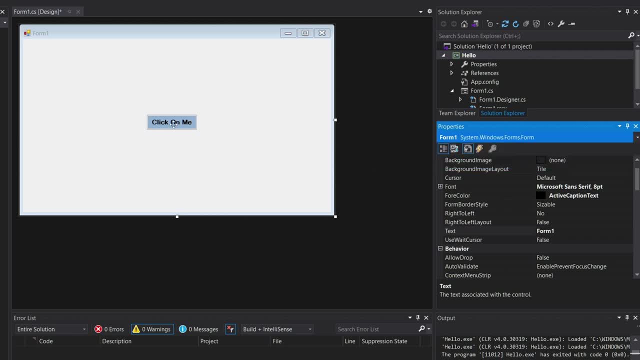 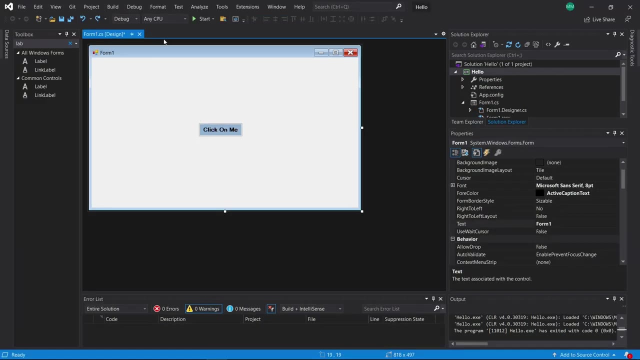 But you can change it. You can select the component from here. Okay, You can check label. You can also change it. You can change its text back. Okay, So let's go back. So now the font doesn't appear. 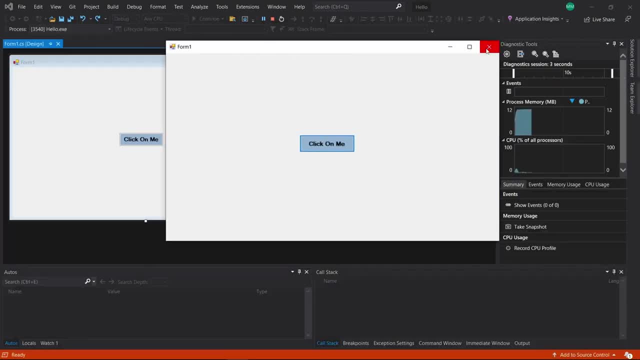 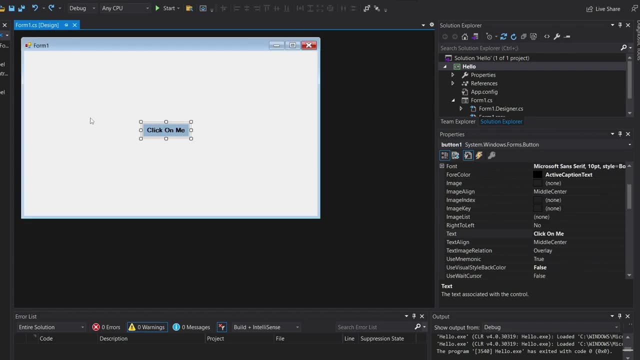 If we run the program, the font does not appear All right. And then after that we want to go to the code And we want to tell the program if the user clicks on the button here. we want you to do something. 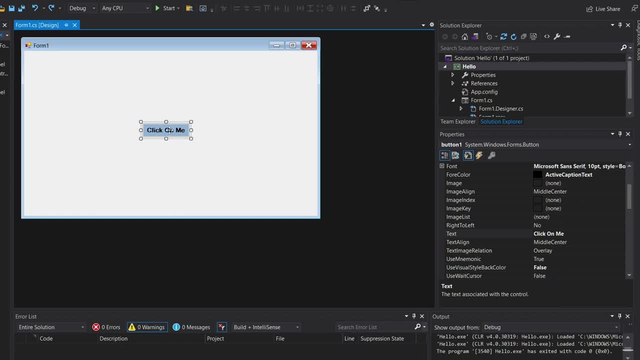 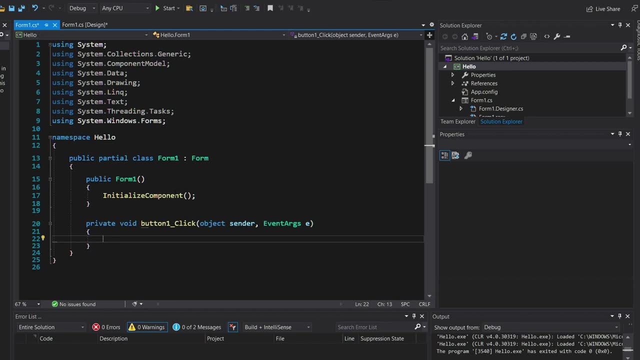 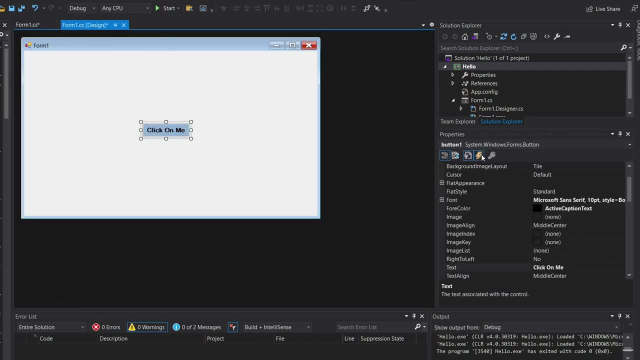 So you can do this in multiple ways. You can double click on this and it will show you the code. here You see Windows Forms. Okay, So this is button one click when you click on the button, Or you can also select it and then go to the events. 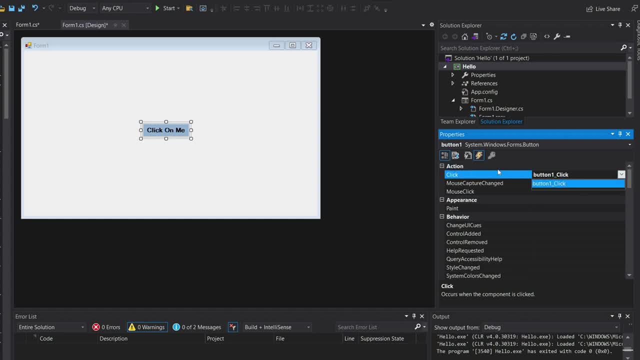 And here in the events tab. you see, In the events tab you can select the click Mouse capture, change Mouse click, Print A lot of things here, So you can just double click on it. Okay, So now go back to the properties tab. 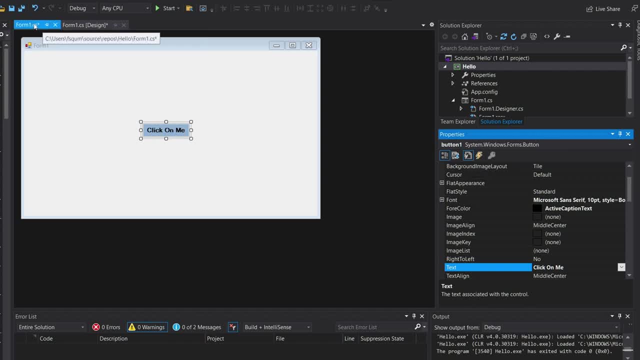 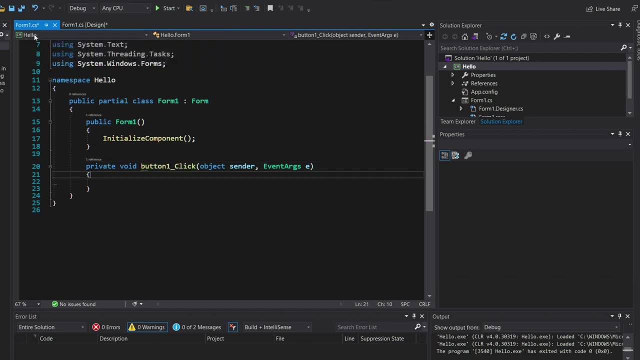 And then now we want to go to the code Here you can see the code will be forms1.cs. Cs means C sharp. Okay, So in forms one, this is the form one. You see, This is the title of the form. 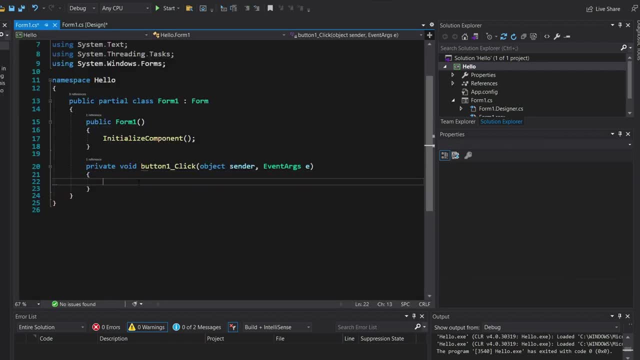 That means the window here, Okay, And we can assign it to do something. So if we click on the button here, we want to change the label one. So label We call the name of the object that we want to change. 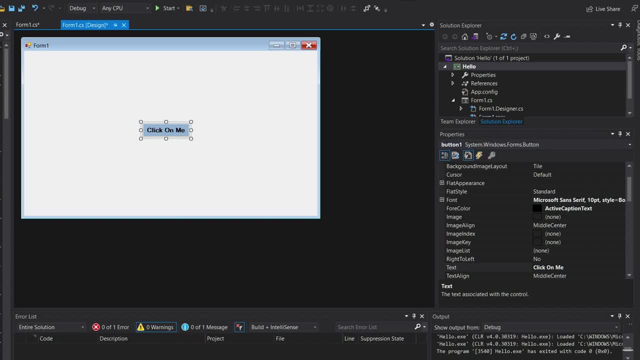 So here the label is here. I have made it. I will keep it with text here. So we want to change this label, So the name of it is here. The name design Name is label one. You can change this. 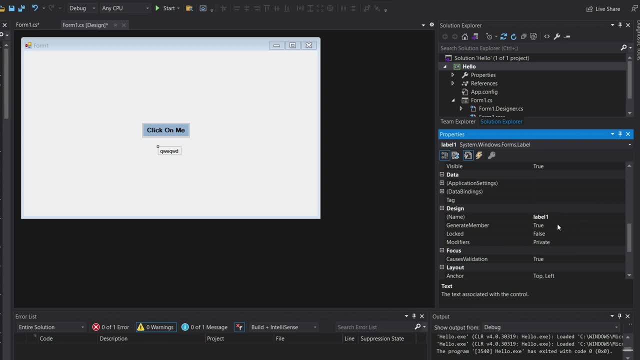 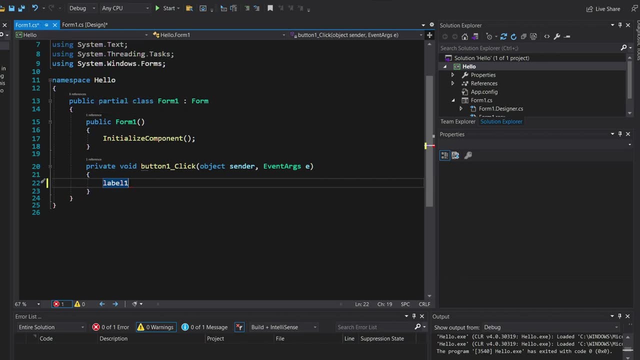 But it's not mandatory. You can change it if you want. I'm not going to change it, I'm just going to keep it the same. So label one dot text. So this will change the text of the label one. 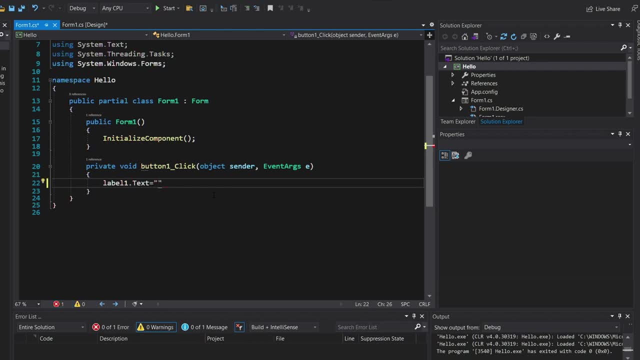 So we will change it to equal to hello. I am a boy And the name of the object is here. So the name of the object is here. So let's change the value and pressure. So this one is all right. 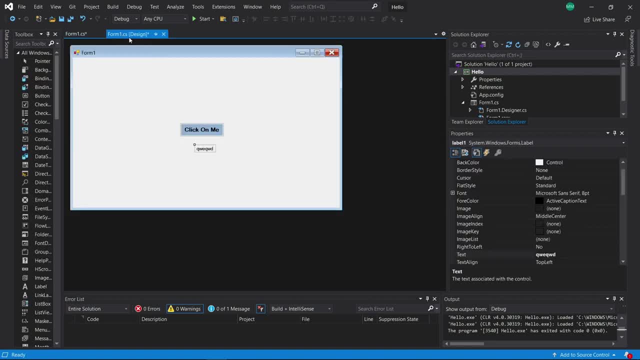 We're going to change the name and we are going to die an object. So now we're going to delete the body, So our hormone will have a yellow color. So now we're going to make the cell the button. Okay. 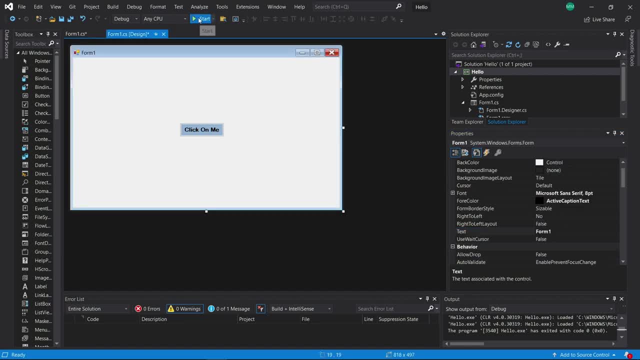 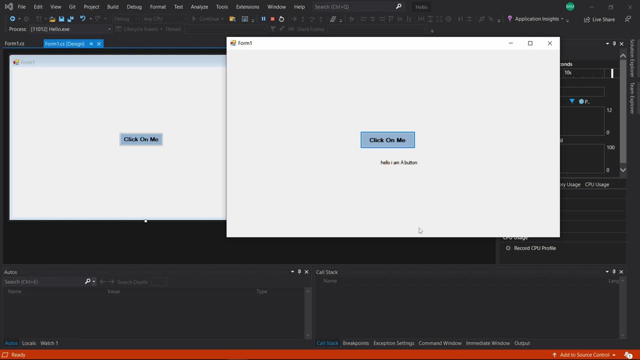 So it will see that it is a button when you click on it. Okay, And that's it. That is how you do that. see, click on me. it will say: hello, i am a button, okay. um, okay, so let's say we wanted to change the. 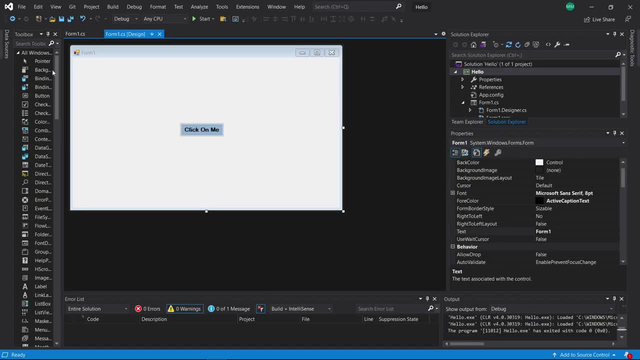 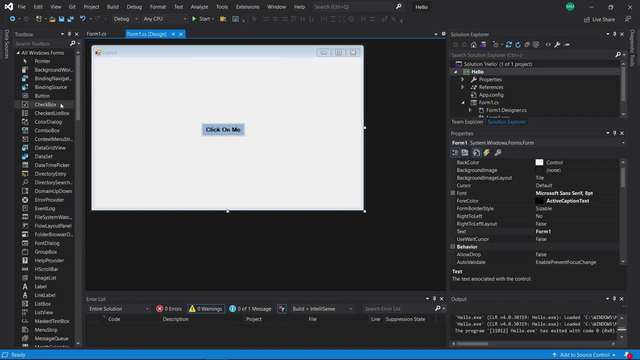 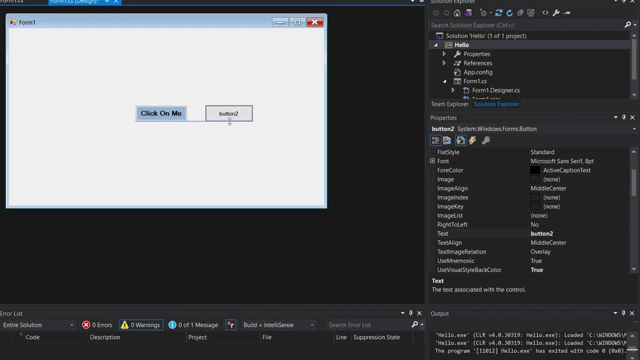 color of this font. so if we wanted to do that, you can. you can do it in multiple ways, but i will check, i will. i will add another button here. we'll add another button. okay, scale it bigger so we can make it the same. okay, all right. and then for button two, we want it to, uh, change the. 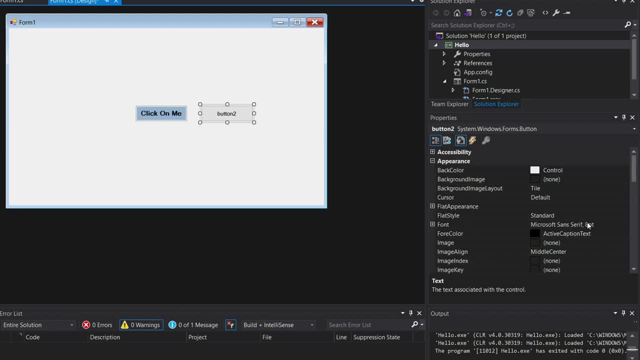 color. so let's change the properties to match this. so go back to the appearance and then go to back color and then change the color from that to this, okay. and then we want to change the text, so go down to text. okay, let's say, change text or change color, okay, so we will change color whenever we press on. 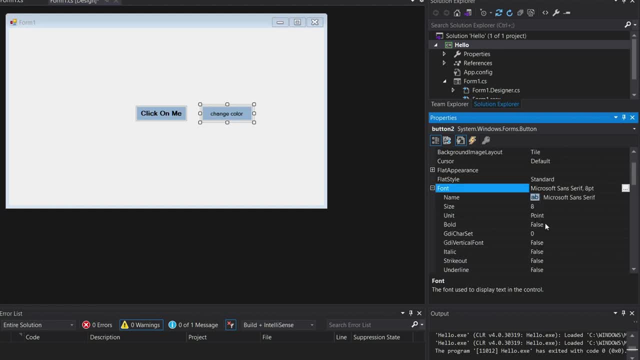 the button. okay, so let's make it bold, so it's more visible. uh, bold, bold, so bold is equal to true, okay. and then we want also to: yeah, let's make it a little bit bigger, so 10, okay, that's pretty good. change color, all right, so now we can also. we can also do the same thing for 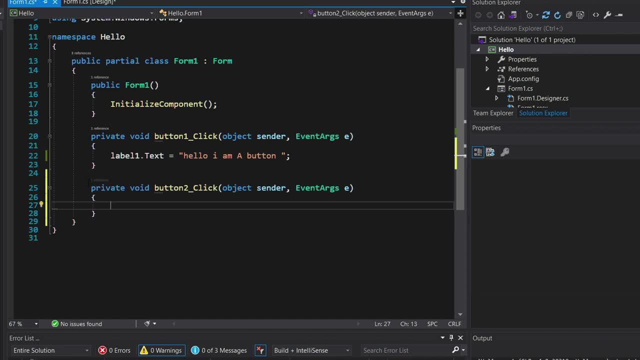 the click. so when we double click on it, you will add, he will, the program will add the code here. so now you can change the, the color of the label one. so label one dot text equals color dot. we will change the color to something else. let's see, uh, let's say blue, okay, so let's make it. 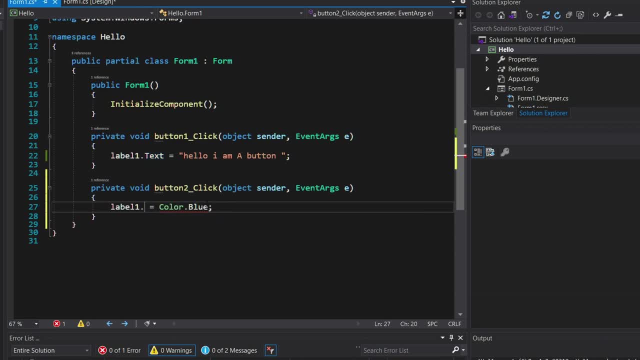 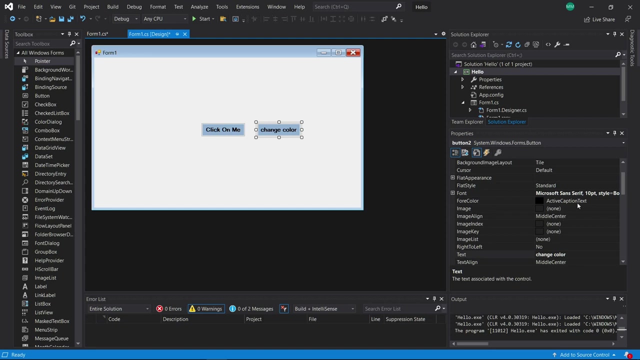 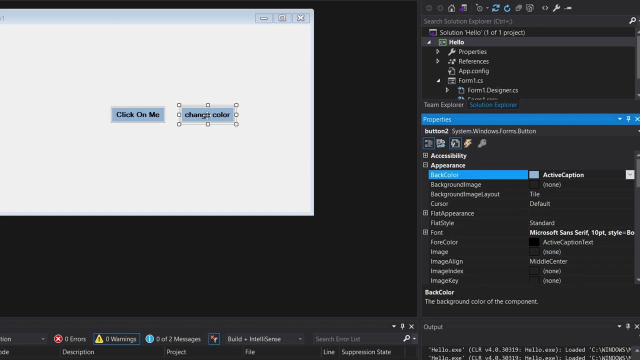 blue and uh four color. we want to change the foreground color, so four color. that will change the color of the foreground here it this will: here you can see, uh four color here this is the background color. you see, and this will be for color. you see, here it will change the font inside of the 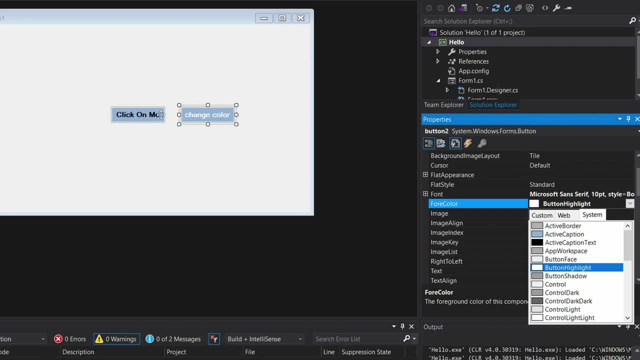 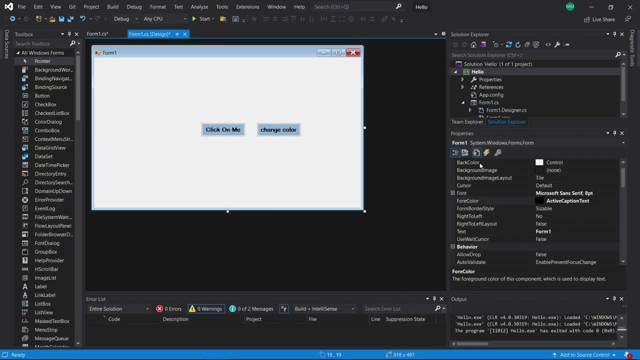 the text. okay, so the foreground color. we want to change the foreground color for the label, um, change it back to black. and now here, this will change the color to blue. okay, so now run the program and, as you can see, click on me so we'll click on the button. hello, i am a button.